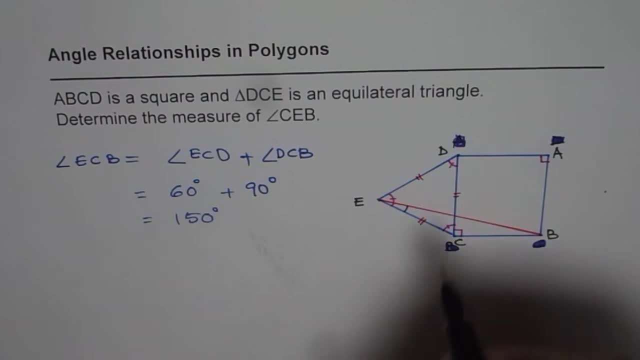 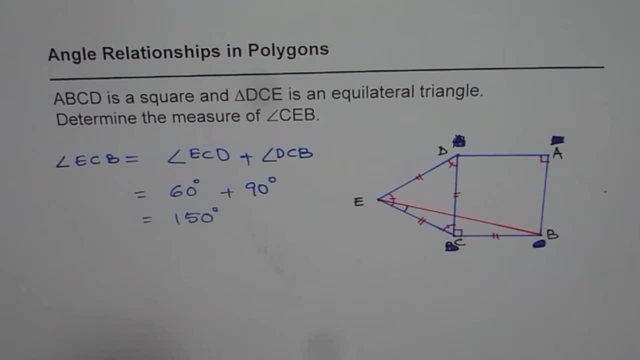 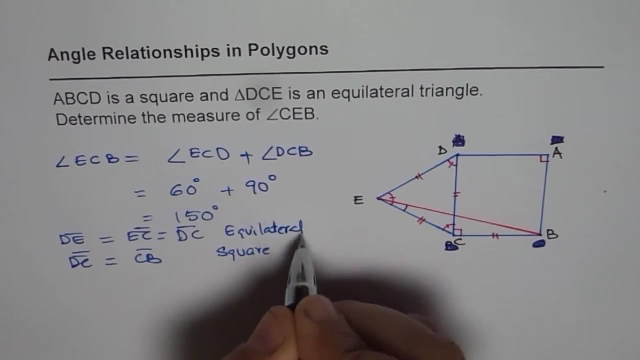 Right, Right, Right, Right, Right is equal to CB, Since these are the sides of a square right, So this is square And that's an equilateral triangle. From here we can say that EC is equal to CB right. 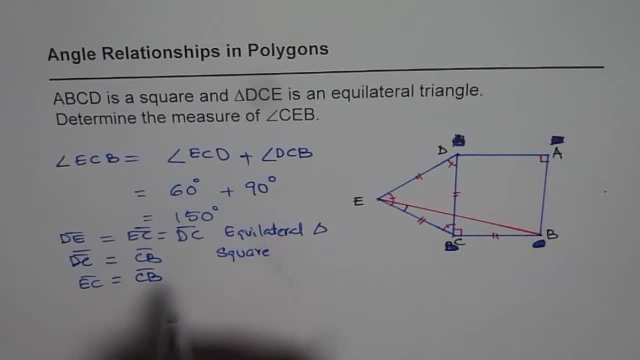 So we have EC equals to CB. They are congruent sides. Now when EC and CB are equal, then that means that the triangle ECB is an isosceles triangle, right, So it's two sides are equal. Now if two sides are equal, then angle BCE, BEC, is congruent to angle EBC, correct? So? 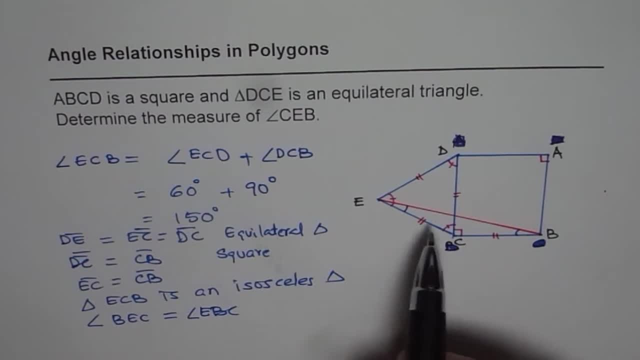 these two angles are equal. Sum of the three angles is 180 degrees, right? Therefore, what we can say is that angle. let me write it down here now. Now, since these two angles are equal, we can say that two times angle BEC plus angle ECB. 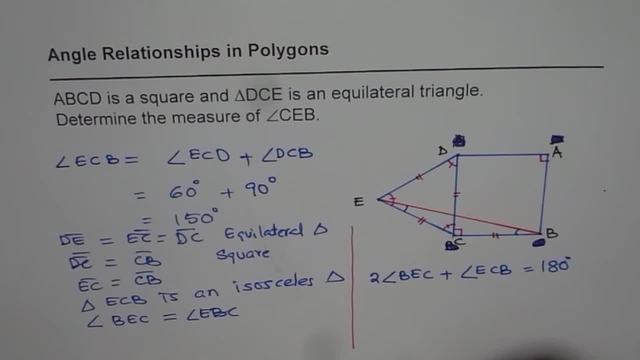 B is equal to 180 degrees, correct. Now angle ECB is known to us as 150.. So two times angle BEC is equal to 180 degrees minus 150 degrees. That is 30 degrees, correct. And therefore angle BEC is equal to 30 degrees divided by 2 or 15 degrees. That is how we can find the